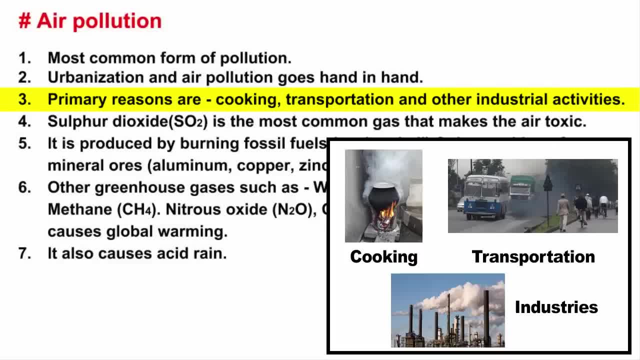 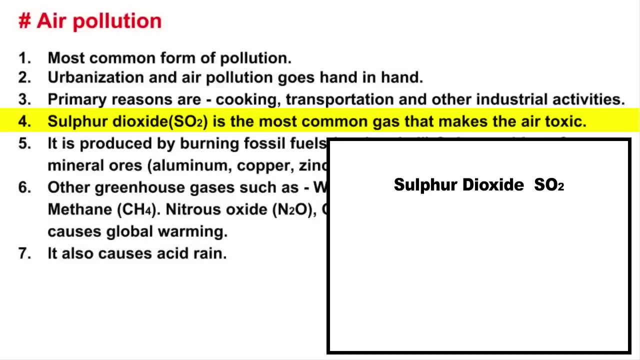 cooking, transportation and other industrial activities can cause air pollution. Air pollution is industrial activities is the primary reason behind air pollution. Sulphur dioxide is the most common gas that is making the air toxic. It is produced from the burning of fossil fuels like coal and oil. 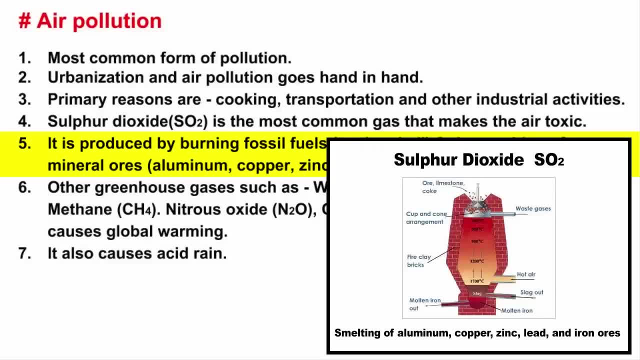 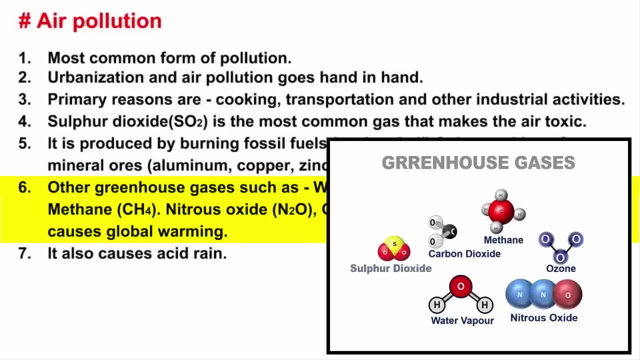 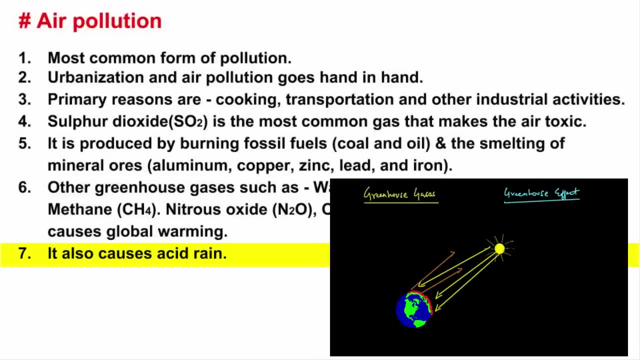 and the smelting of mineral ores like aluminium, copper, zinc, lead and iron. The release of sulphur dioxide and other greenhouse gases into air causes global warming and has capacity to cause acid rain. I have a separate video on how greenhouse gases can cause global warming, If you. 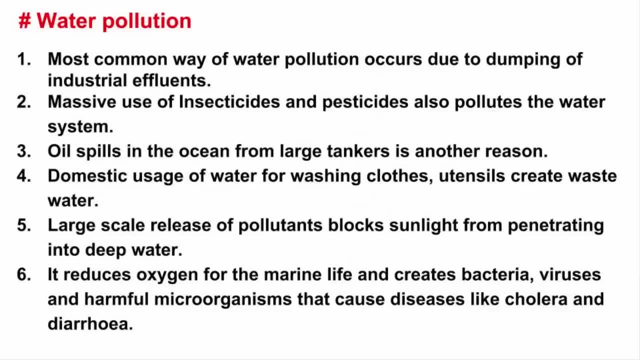 want to have a look at it. I'll put the link in the description. The second one is water pollution. Every living being on earth depends on water for its survival. Thus, water pollution is another major type of pollution. Industrial effluent dumped into the rivers and sea is the most common. 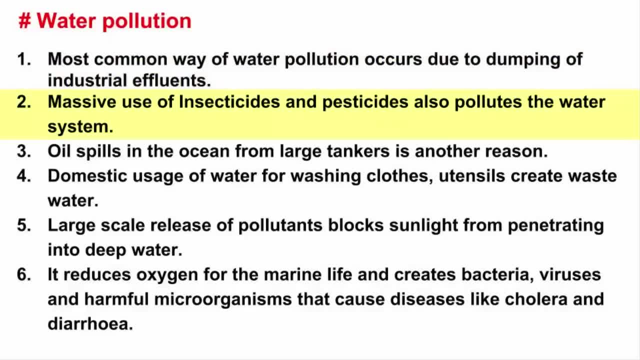 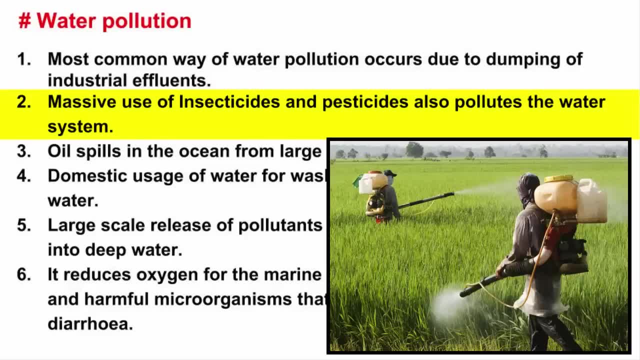 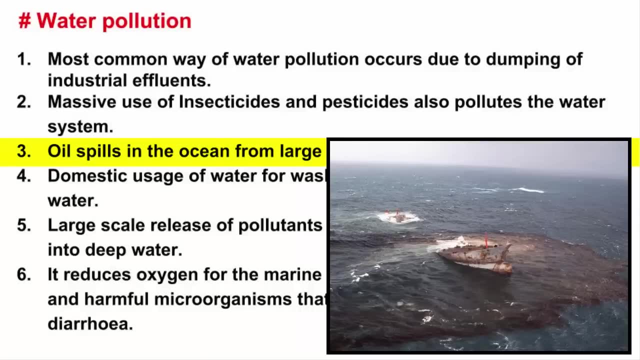 way in which water is getting polluted. After that, the massive use of insecticides and pesticides by agricultural community is polluting the ground as well as the water system. Then oil spills in the oceans by the heavy tankers have caused significant damage to the water bodies. Then 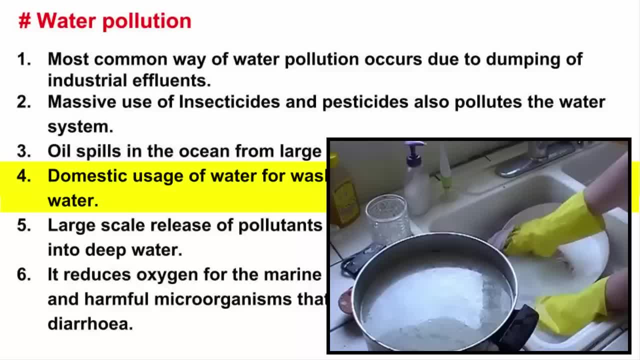 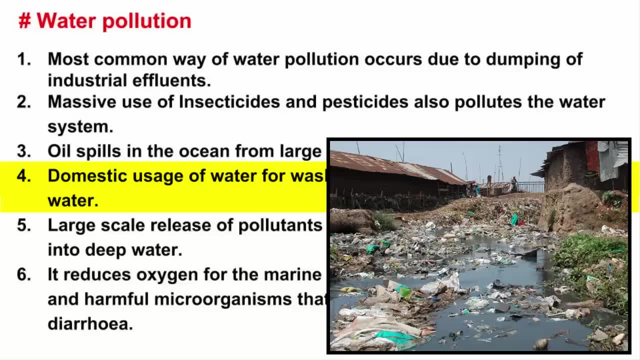 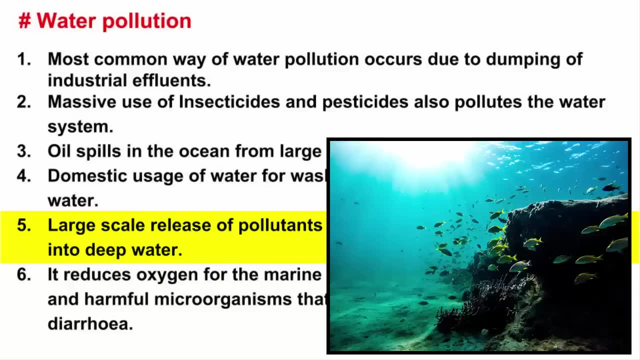 washing clothes utensils create waste water. With no proper sewage treatment, these waste water are released directly into ponds and lakes, which causes heavy water pollution. The whole point behind all of this is, when large-scale pollutants are released into the water, it blocks sunlight from penetrating, thus reducing oxygen from the marine life, and it also changes. 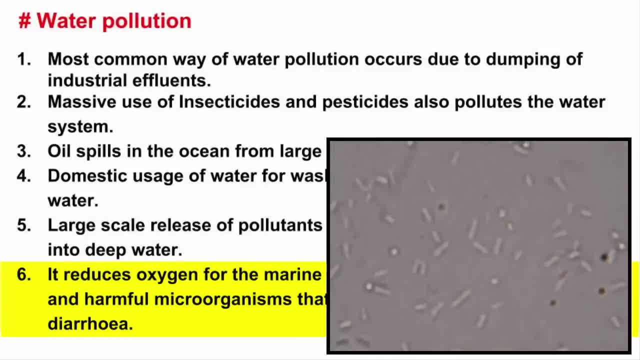 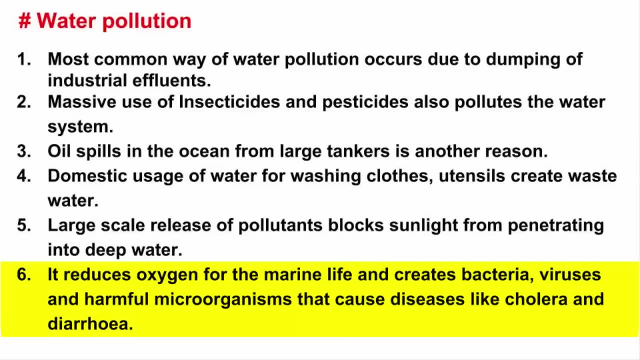 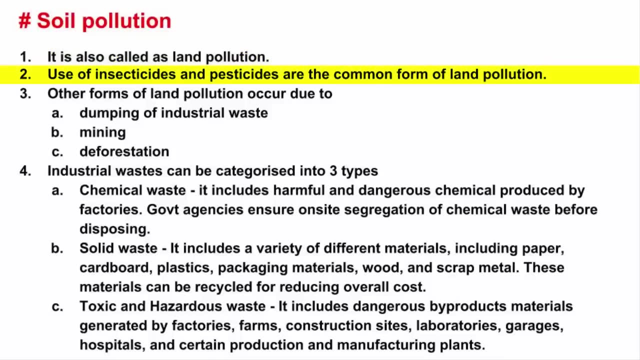 their composition due to the introduction of new forms of bacteria, viruses and other microorganisms that can cause water-borne diseases like cholera and diarrhea. The third one is soil pollution. This can also be called as land pollution, The most common form of land pollutant. you can think. 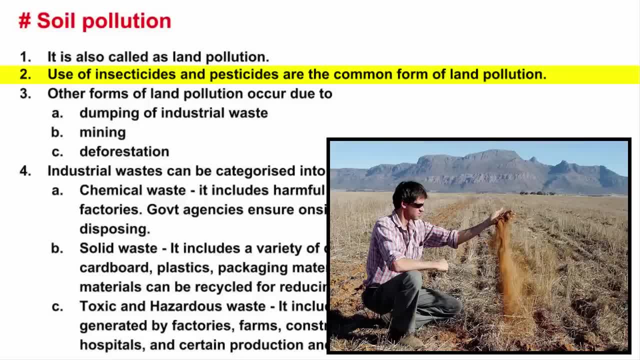 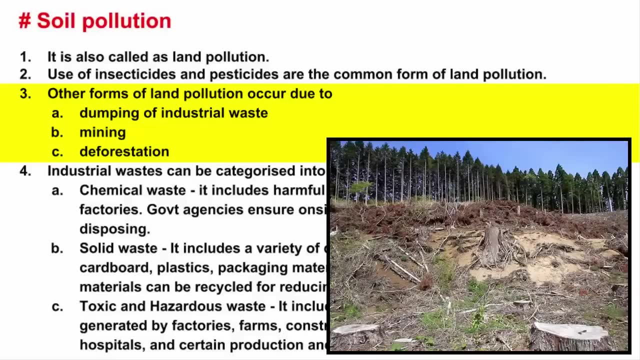 of is the use of insecticides and pesticides. The use of these chemicals can lead to exhaustion of the nitrogen compounds from the soil, making it unfit for plants to grow. Other forms of land pollution occur due to dumping of industrial waste, mining and deforestation. Industrial waste can be categorized into three types. 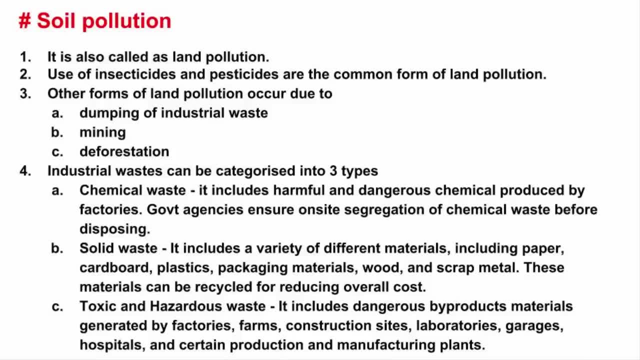 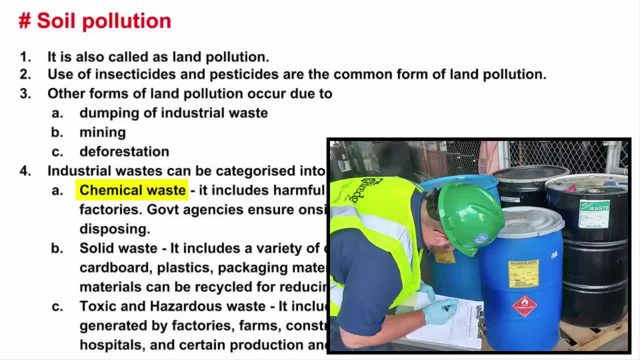 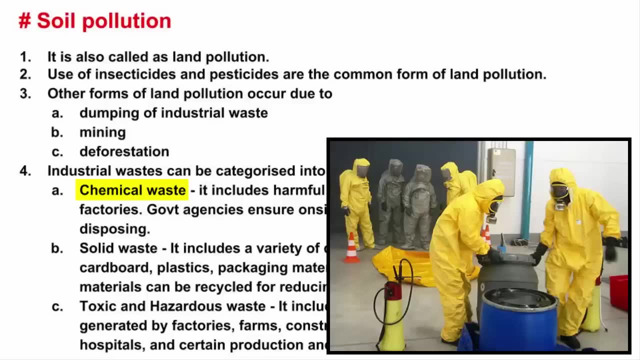 chemical waste, solid waste and toxic and hazardous waste. Chemical waste includes harmful and dangerous chemicals which are typically generated by factories. There are rules and regulations made by the Government and Environmental agencies which ensure that chemical waste must be supergated onsite and disposed on site. 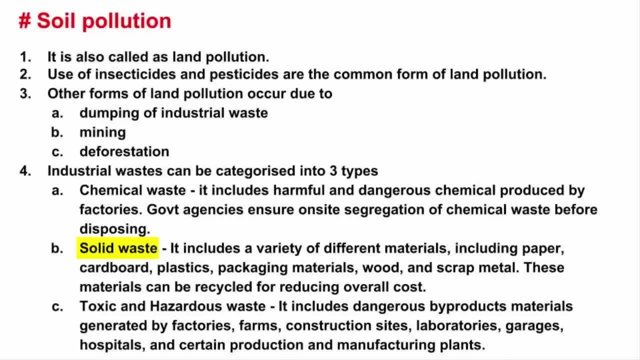 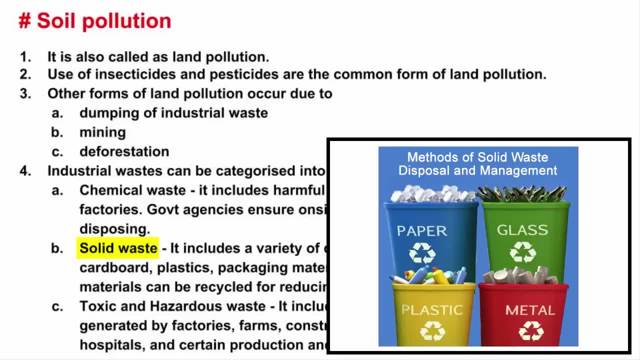 Now, what are solid wastes? In industrial services, solid waste include a variety of different materials, including paper, plastic, cardboard, packaging materials, spare materials, wood and scrap metal. Some of these materials can be r-used and repulsed from the recycling center. 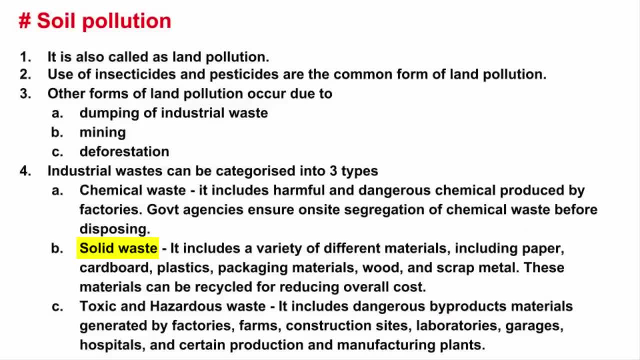 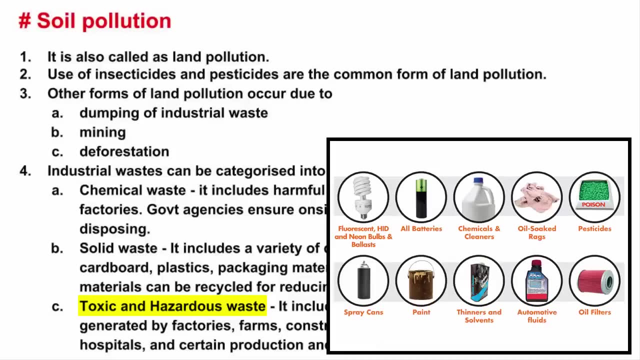 Recycling is important because: ● it effectively reduces em, WOMAN, in�� your waste disposal cost. Then toxic and hazardous waste. It comprises of materials that can cause serious health and safety problems if waste disposal is not handled correctly. This type of waste typically includes dangerous by-product. 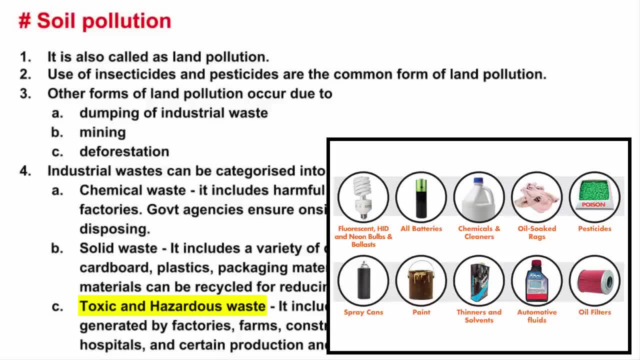 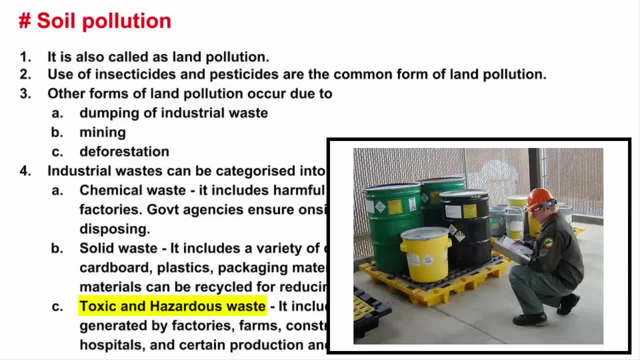 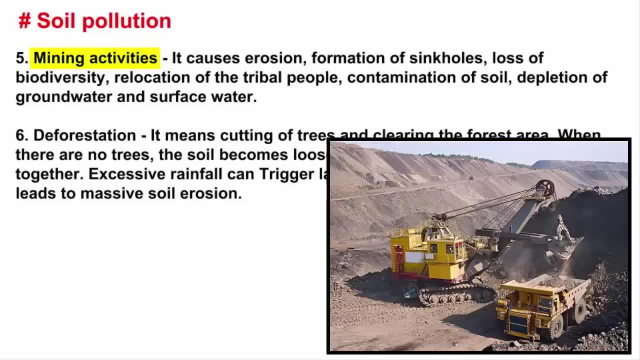 materials generated by factories, farms, construction sites, laboratories, garages, hospitals and certain production and manufacturing plants. This waste disposal is only legal at special designated facilities around the country. Now, mining activities like excavation, overburden, dumping has some serious environmental 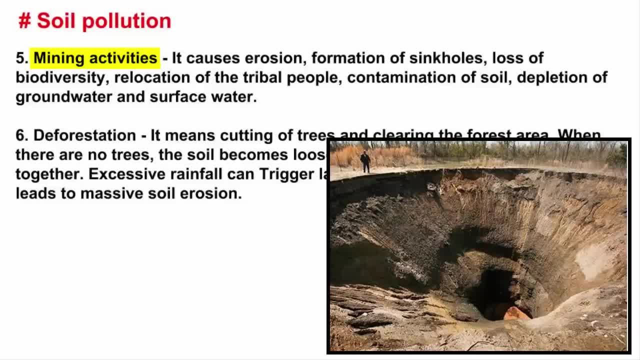 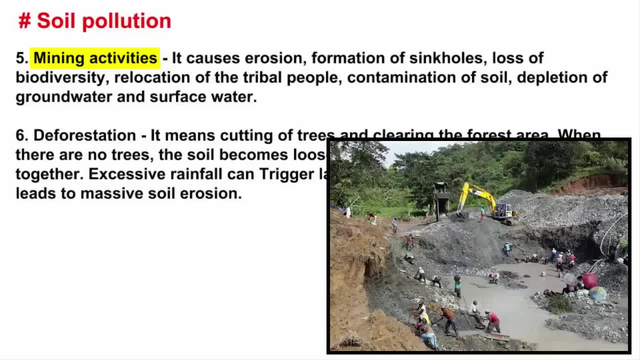 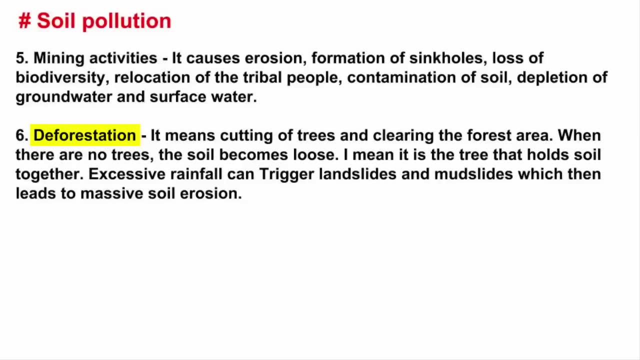 impact, which include erosion, formation of sinkholes, loss of biodiversity, relocation of the tribal people, contamination of soil, depletion of groundwater and surface water. Deforestation means cutting of trees and clearing the forest area. When there are no trees, the soil becomes loose. 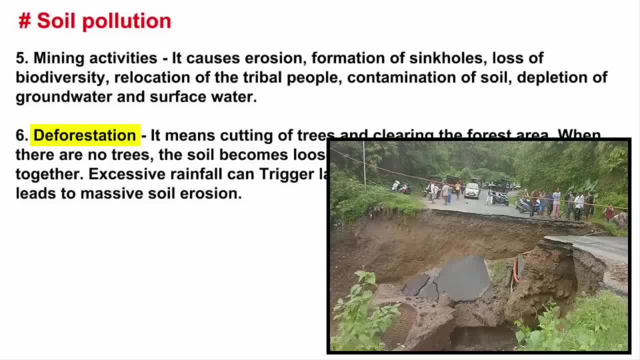 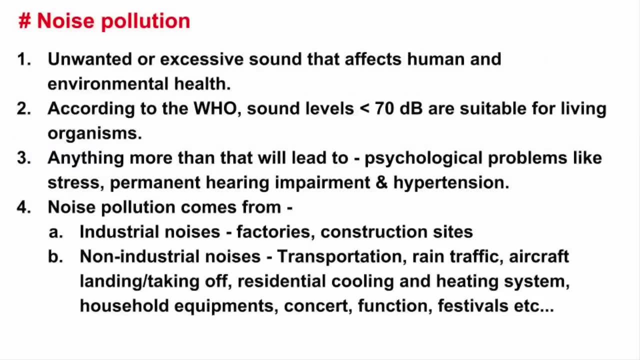 Deforestation means cutting of trees and clearing the forest area. When there are no trees, the soil becomes loose. I mean, it is the tree that holds the soil together. Excessive rainfall can trigger landslides and mudslides, which then leads to massive soil erosion. The fourth: 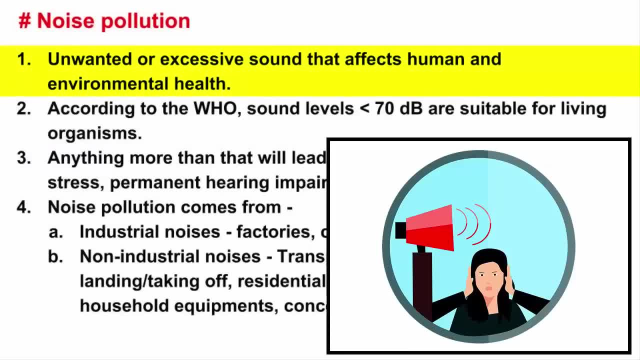 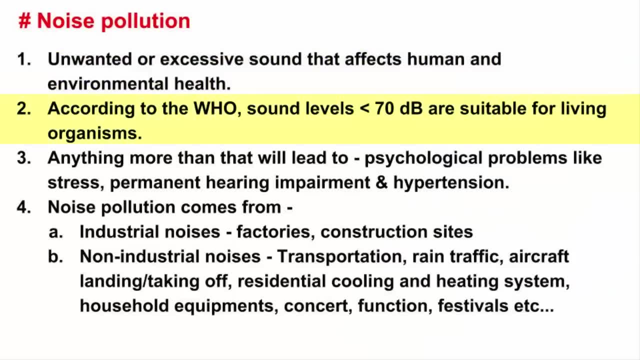 one is noise pollution. Unwanted or excessive sound that can have serious effects on human as well as environmental health leads to noise pollution. According to the World Health Organization, sound levels less than 70 decibel are not damaging to living organisms. Anything more than that may. 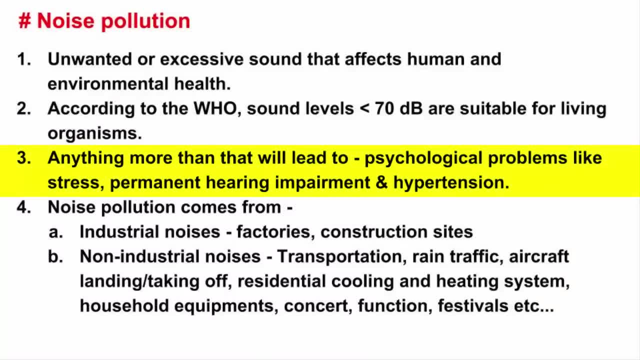 lead to psychological problems like stress, permanent hearing impairment and hypertension. Noise pollution comes from factories, ie operations of machines and motors. It comes from construction sites, like operations of cranes and welding. These all fall under industrial noise. There are non-industrial noises as well, such as transportation, road traffic, honking. 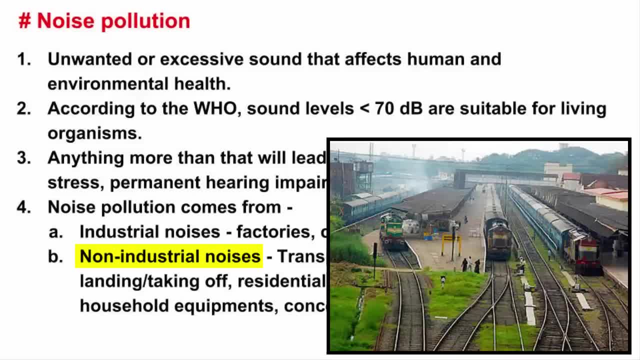 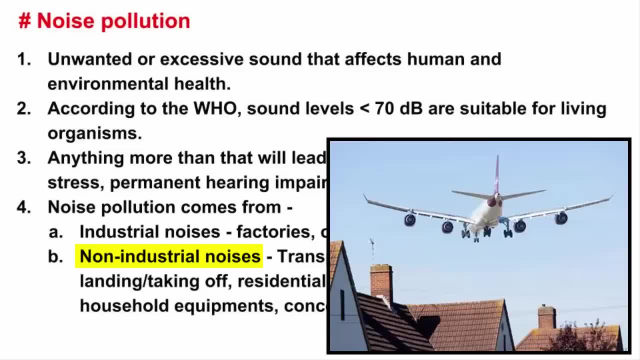 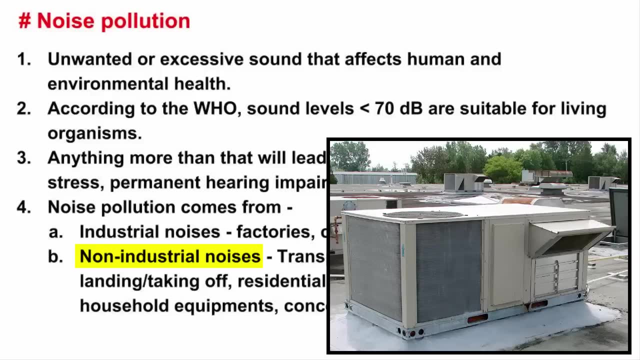 and the vehicle engine noise. transactional noise also causes noise from the train wheels and engine, then noise coming from aircraft taking off and landing In residential areas. noise pollution is caused due to cooling and heating systems, then household equipment, then community concert festival, etc. 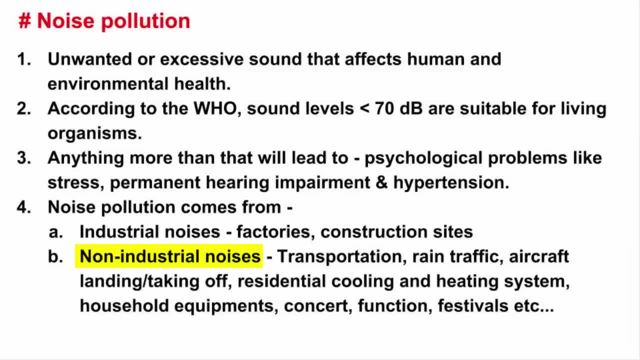 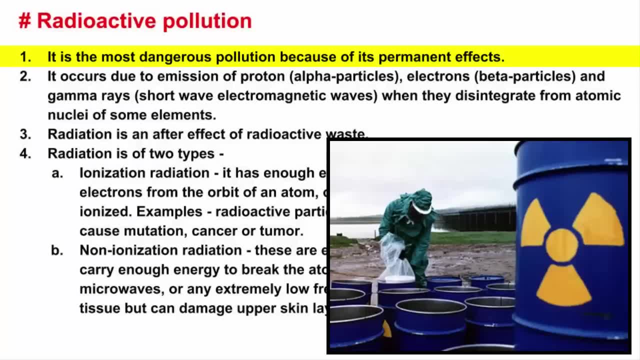 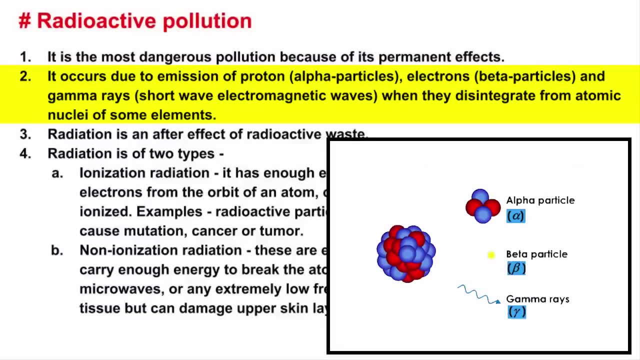 All of this comes under non-industrial noise. The fifth one is radioactive pollution. This is considered one of the most dangerous pollution because of its permanent effects. Now, radioactive pollution occurs due to emission of proton, which are alpha particles, then electrons, which are beta particles, and gamma rays, which are short wave electromagnetic. 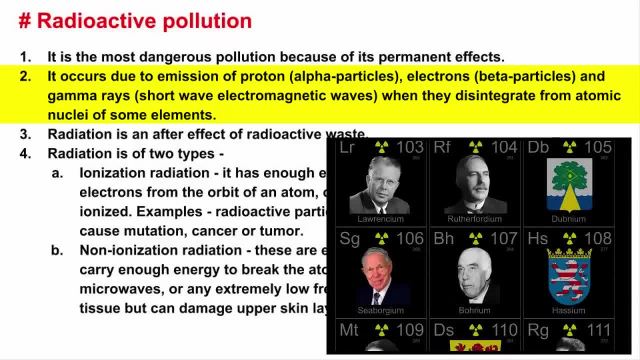 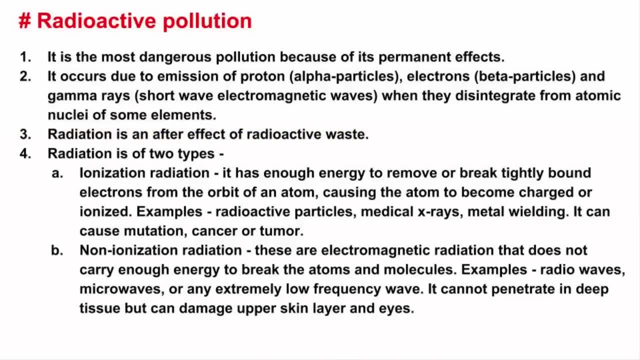 waves when they disintegrate from atomic nuclei of some elements. Now radiation is an aftereffect of radioactive waste. Radiation can be categorized into two groups: non-ionizing radiation and ionizing radiation. Ionizing radiation has enough energy so that during an incident, radiation can be released. 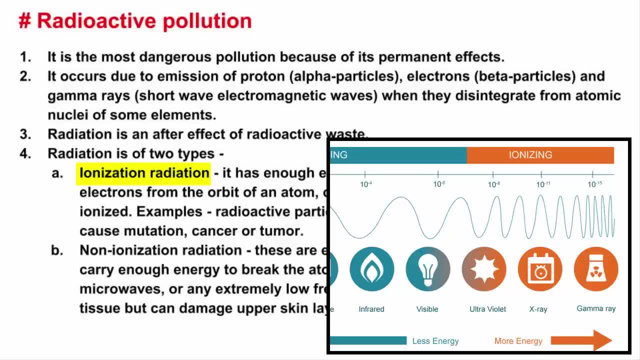 During an interaction with an atom. it can remove or break tightly bound electrons from the orbit of an atom, causing the atom to become charged or ionized. Some examples of ionizing radiation are radioactive particles, then medical x-rays, then metal welding. 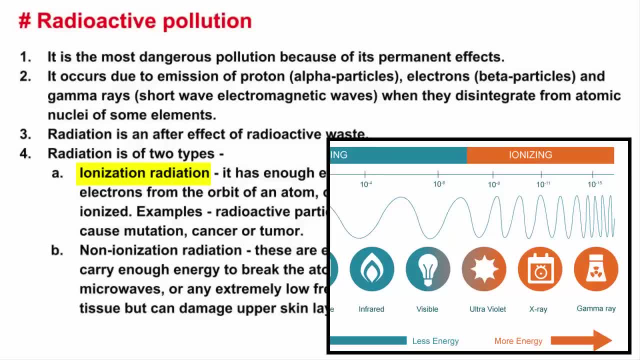 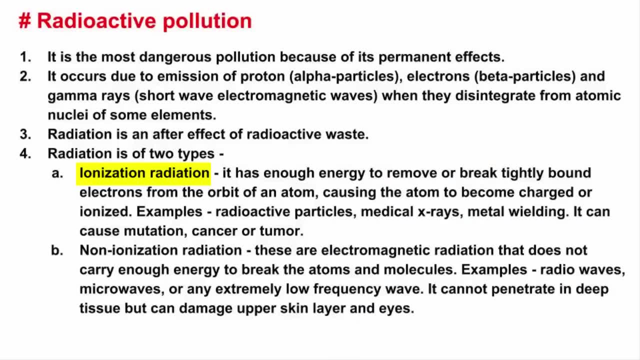 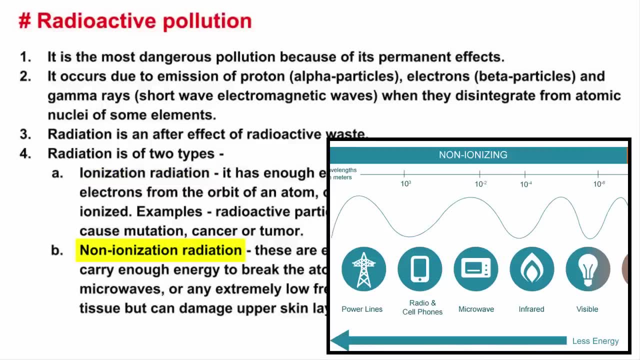 If human body is exposed to ionizing radiation, it can break bonds in proteins and other important molecules in our body and that can cause mutation, cancer or tumor Which can lead to death. Now, non-ionizing radiation refers to any type of electromagnetic radiation that does not 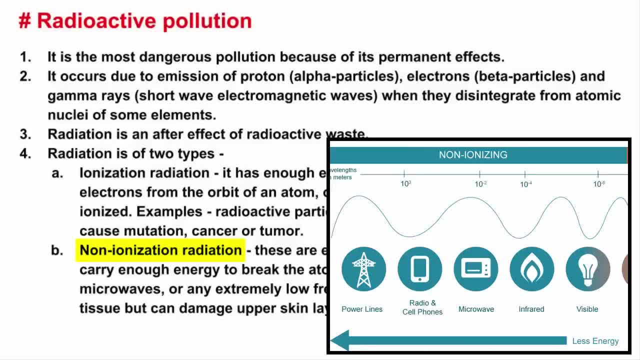 carry enough energy to break the atoms and molecules. Some examples of non-ionizing radiation are radio waves, microwaves or any extremely low frequency wave. Non-ionizing radiation does not penetrate deep into the tissues, but it can damage the upper skin layer and eyes. 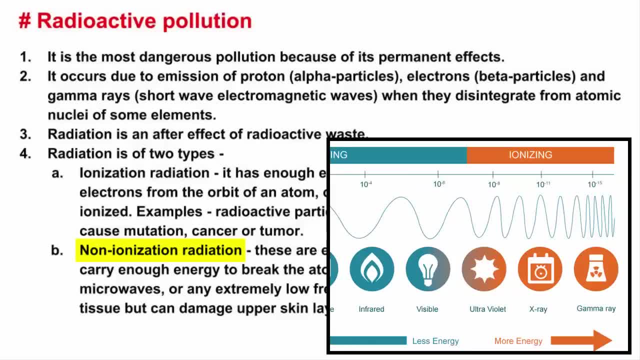 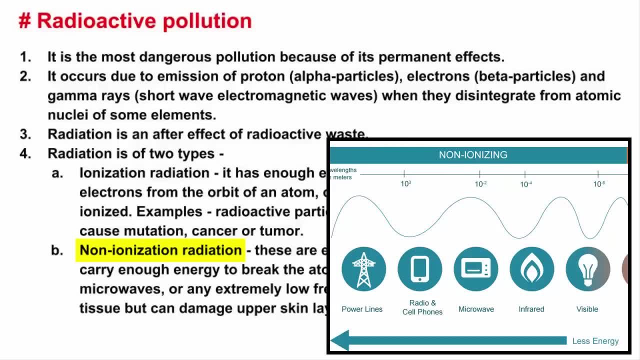 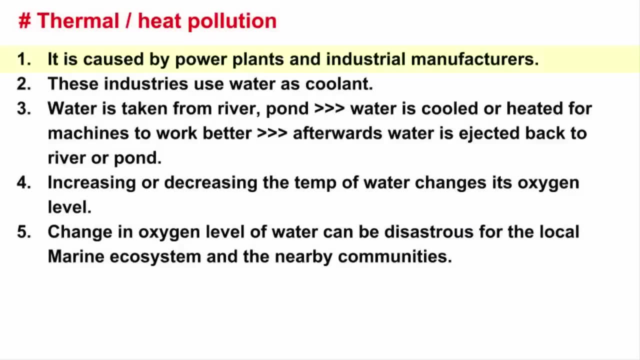 So the point is: Ionizing radiation have a lot of energy to penetrate and break bonds. On the other hand, non-ionizing radiations do not have enough energy to penetrate and break bonds. The fifth one is thermal or heat pollution. Thermal pollution is commonly caused by power plants and industrial manufacturers.